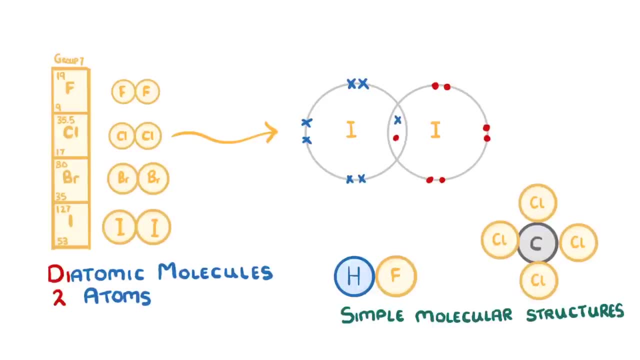 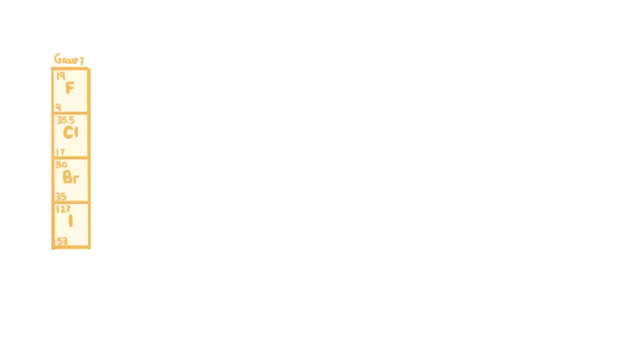 are known as simple molecular structures and we take a closer look at them and the covalent bonds they use in another video. Just like the group 1, elements, group 7 also has trends as you go down the group, but they're. 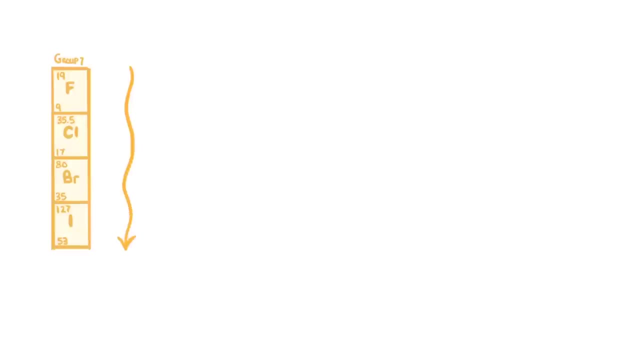 the opposite way around. For halogens, the melting points and boiling points increase as you go down the group and the reactivity decreases. So for halogens, they have more of a covalent bond and a boiling point, so the reactivity decreases. For halogens, the 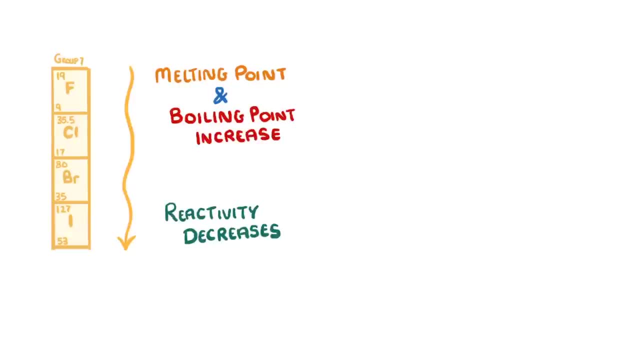 reactivity decreases. This decrease in reactivity is because as you go down the group, the outermost shell gets further and further away from the positive nucleus. So the attractive force that's needed to pull in an extra electron from another atom gets weaker. And if the 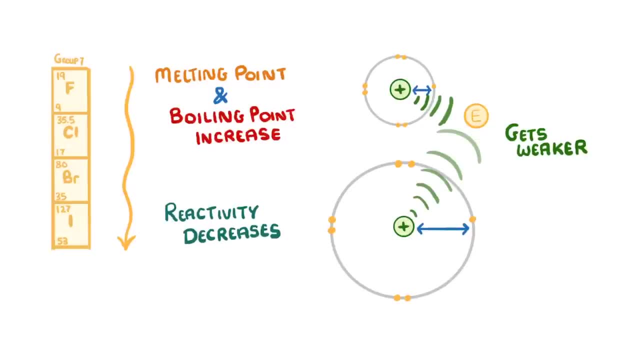 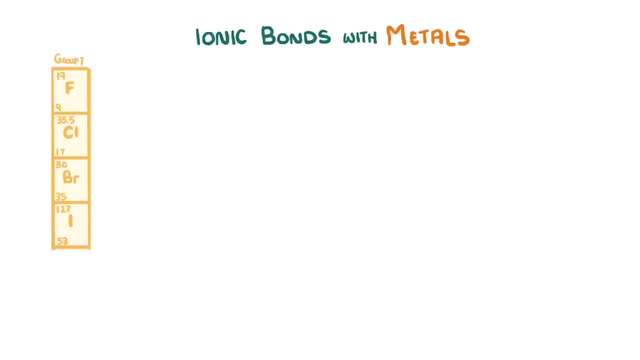 halogen can't attract an electron to complete its outer shell, then it can't react. So the larger atoms at the bottom of the table, like iodine, are the least reactive. The next thing we need to look at is how halogens form ionic bonds with metals. When a halogen 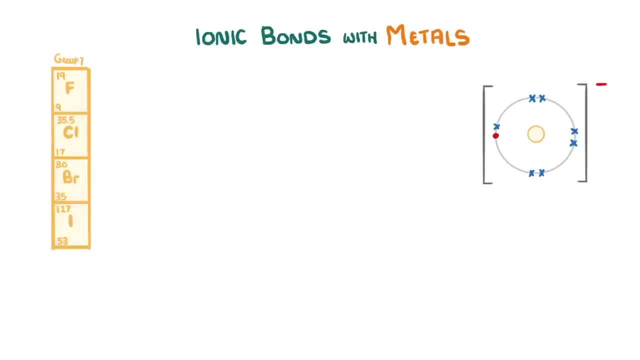 gains an electron to form a 1- ion. we call it a halide and we have to change the name slightly, changing the n's to d's, So we get fluoride, chloride, bromide and iodide, all of which would be ions. 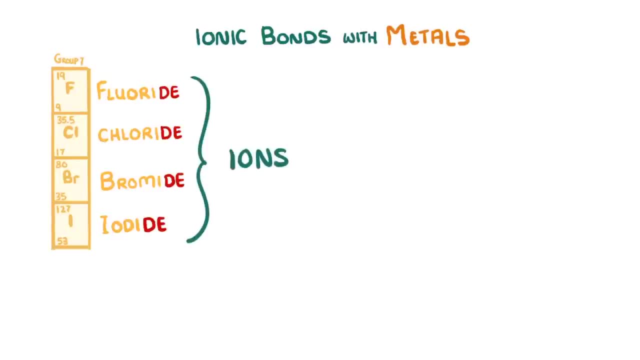 You will probably most often see halogens forming ionic compounds with the alkali metals in group 1, like sodium chloride, as we have here, but they can form ionic bonds with metals of other groups too. Lastly, we need to take a look at displacement reactions. These involve a more reactive halogen. 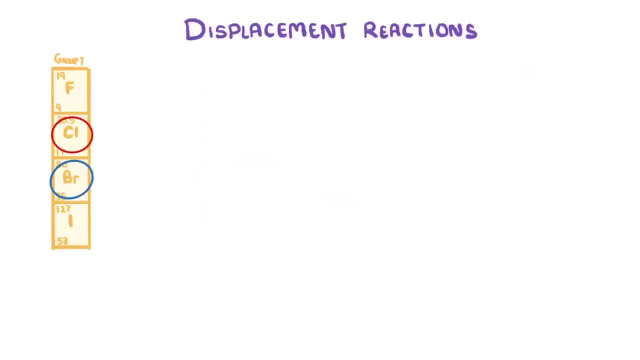 displacing a less reactive one. For example, let's imagine that we pumped some chlorine gas into a solution of potassium bromide. As the chlorine is more reactive than the bromine because it's higher up in the group, it displaces the bromide to bond to the potassium So effectively the chlorine has taken the.